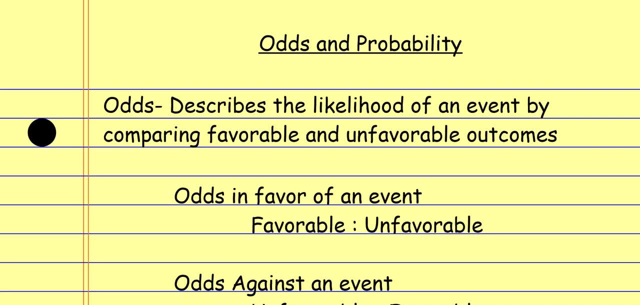 over the total number of outcomes. And odds is very similar to that, but instead of describing the likelihood in terms of the total number of possibilities, we describe the likelihood based on favorable versus unfavorable. okay, So odds describes the likelihood of an event by comparing the favorable and unfavorable outcomes, And again, that's a very slight 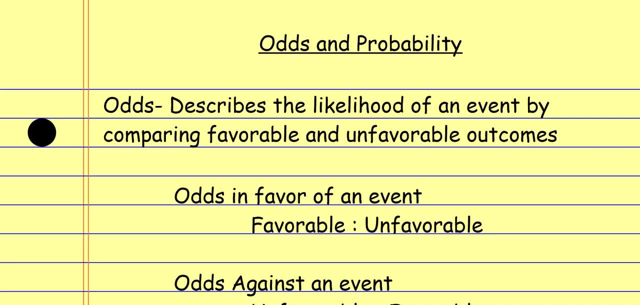 difference from probability. Probability was favorable versus the total. Odds is favorable versus unfavorable. So odds in favor of an event, we list the favorable first and then we list the unfavorable And we list it in kind of this ratio type of format. 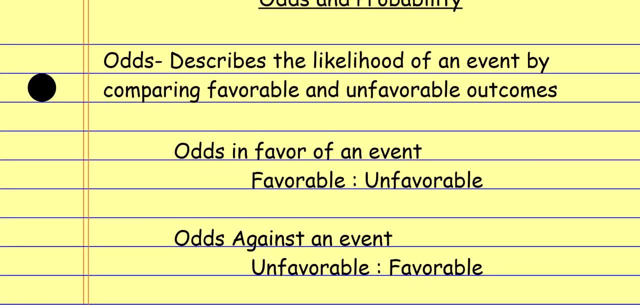 And this is the same thing as expressing a fraction, but really we don't express it as a fraction so that we don't get it confused with probability. So if the favorable to unfavorable was one to two, instead of writing one over two, we want to write one and then a colon and then a. 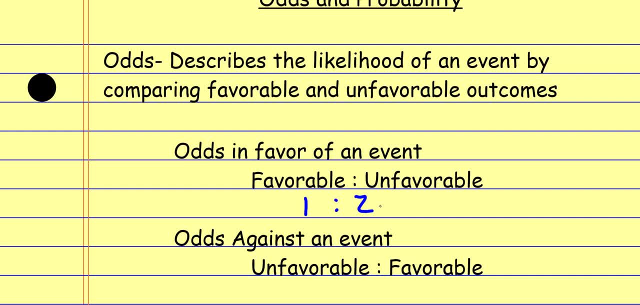 two. It's the same as writing a fraction, but it's just a different way of expressing that ratio. okay, Odds against an event. basically, we just flip those around. So I list the unfavorable first and then the favorable. okay And again, instead of doing what we want over the total. 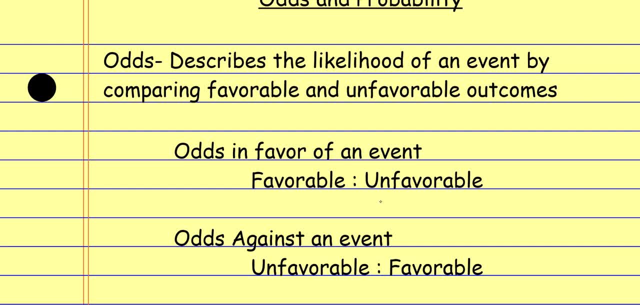 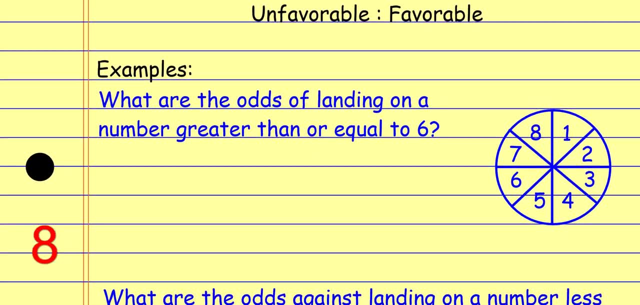 it's what we want versus what we don't want, And then odds against is what we don't want versus what we do want. We just switch the order, okay. For example, here it says: what are the odds of landing on a number greater than or equal to six? So 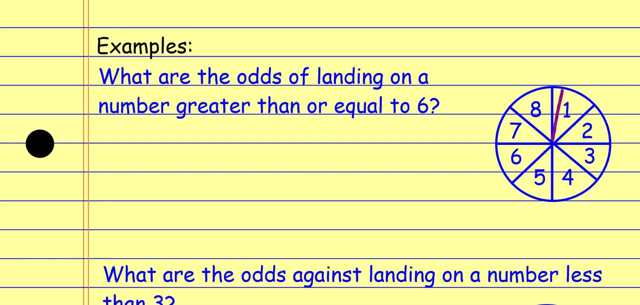 in this scenario. think of this like a spinner, like we've got a little thing on here and we flick it and it spins around, all right. And then we flip it and it spins around, all right, And then it lands on one of these guys- all right. That's the situation that we're talking about here. 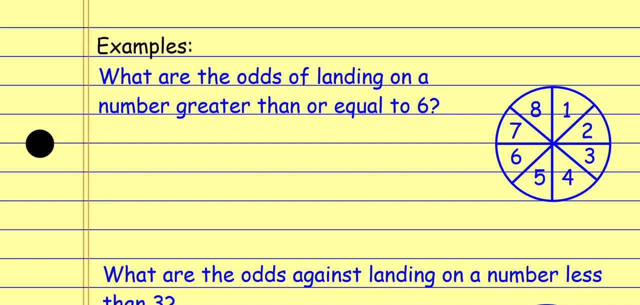 And so if I flick that spinner, the odds of it landing on a number greater than or equal to six, so numbers that are greater than or equal to six would be the six, the seven and the eight. And so if we were to think of this for a second, if we think about probability of the event, 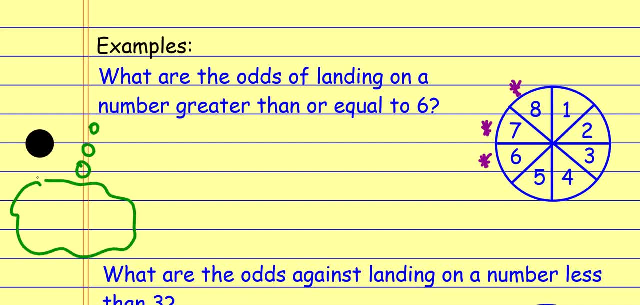 so let me just think about probability for a second, just to show you the difference. So the probability that the number is greater than or equal to six would be three out of the total number of possibilities, which would be eight. okay, But odds are slightly different. We say the odds, we still start with the three. 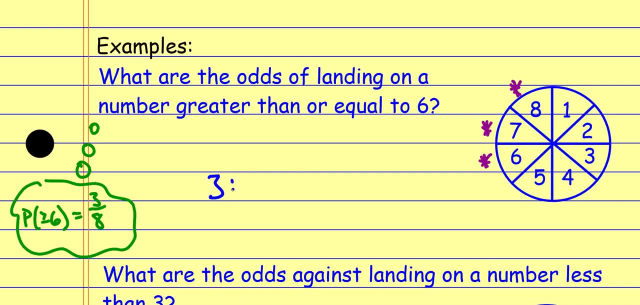 there's three ways that I can get what I want. But then, instead of saying there's three ways I can get what I want over the total of eight, we say, if there's three ways I can get what I want, what's left is that there are one, two, three, four, five ways that I could get something that I 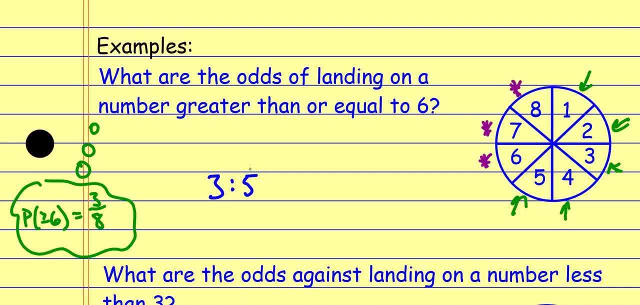 don't want, And so if I flick that spinner, the odds are greater than or equal to six. okay, So the odds are three to five. okay, That's the slight difference here. Instead of saying three out of the total, we say three versus the other stuff. It's three to five instead of three. 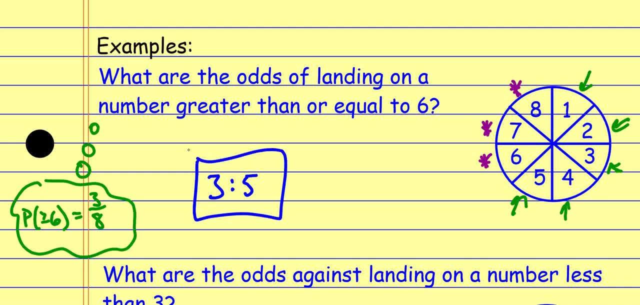 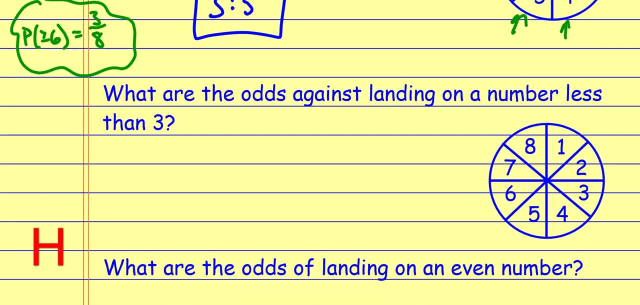 out of eight. okay, That's the slight difference between odds and probability. all right, Using a similar example. so we've got our spinner all set up again. What are the odds against landing on a number less than three? So numbers that are less than three would be the two. 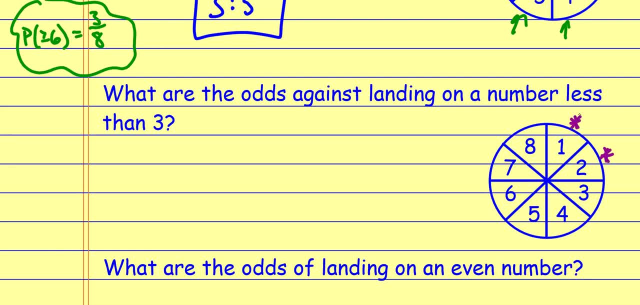 and the one: Okay. So the odds of landing on a number less than three would be two to six, because there's two ways I can get what I want and six ways that I could get something other than what I want. But this says odds against, so I list the unfavorable first. So I just list it as six to two instead. 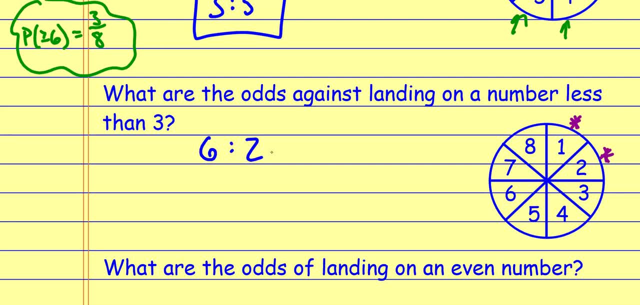 okay, So odds of landing on a number less than three would be two to six. Odds against that would be six to two. I just flip it around, But now, because I could express this as a fraction, I have to reduce it just like I would a fraction. Each of these are divisible by two, So I rewrite it. 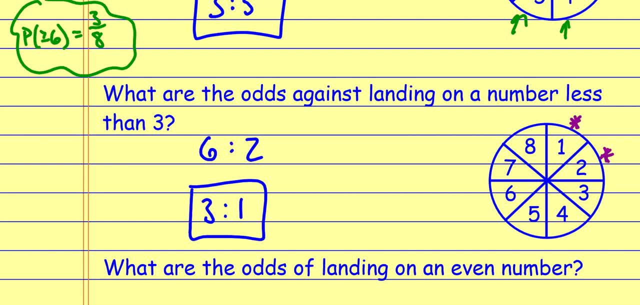 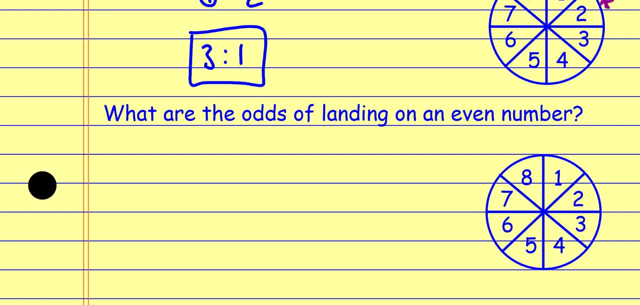 as three to one. okay, Again, a very slight difference between odds and probability. all right, This one. what are the odds of landing on an even number? So I need to count up all the even numbers. We've got this guy, this guy, this one and this one. So the odds of landing on an? 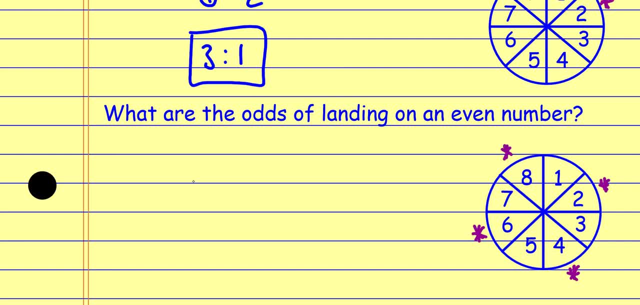 even number would be four. There's four of those. The odds of anything else occurring, of not landing on an even number, would it be everything else? Would it be these four that are left? So the odds of landing on an even number are four to four. 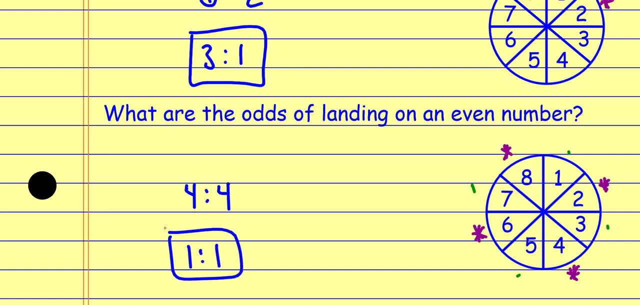 When I reduce it it's one to one, okay. And when we talk about odds, like here, we'd say the odds of landing on an even number are even So. when there's just as likely of a possibility of getting what I want versus what I don't want, we say the odds are even So one to one. or when the odds 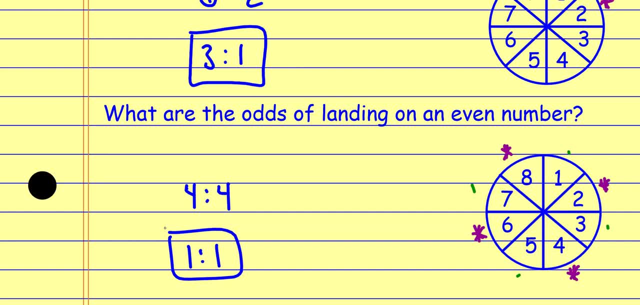 are even. really. what that is showing is that the odds of landing on an even number are even. So what it's showing us is it's showing us, because the odds are one to one, that the probability of getting what I want versus getting something that I don't want are the same. okay, And so odds give. 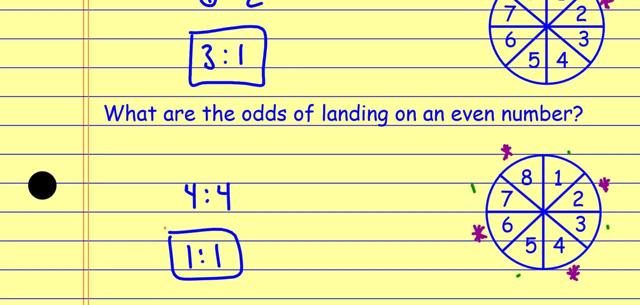 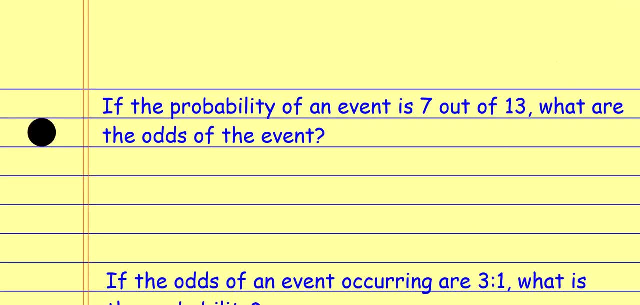 us more of a comparison of the probabilities than they do actually give us probabilities themselves, all right, Favorable versus unfavorable. In this one, we want to know if the probability of an event is seven out of 13,. what are the odds of the event? So again we got to kind of think about. 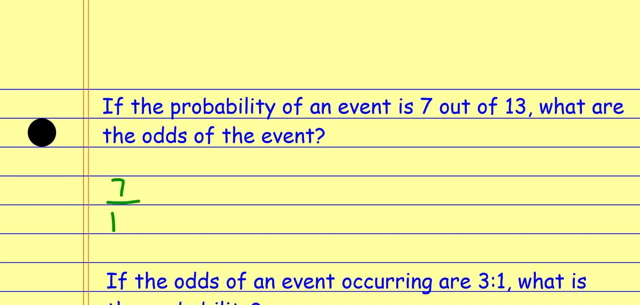 what probability is all right. So when we think about probability, that's seven over 13.. This is the favorable outcomes, right, That's what I want And this is the total number of outcomes. okay, So as we start to think about converting that to odds, remember odds isn't favorable in total. 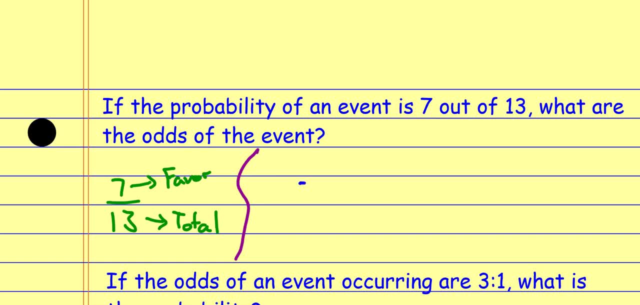 it's favorable versus unfavorable. So the odds of this event would be seven, because that's the favorable outcomes. But now I have to think about it. If there's seven favorable outcomes and there's 13 total outcomes, then I have to think about how I'm going to convert that to odds. 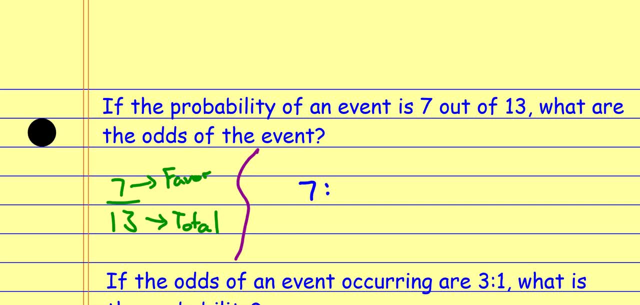 That means there are six outcomes that don't give me what I want. So this would be seven to six, okay. So we have to kind of think about these. things literally mean, If there's 13 total options, seven of them are what I want, that means there's six that give me something that I don't. 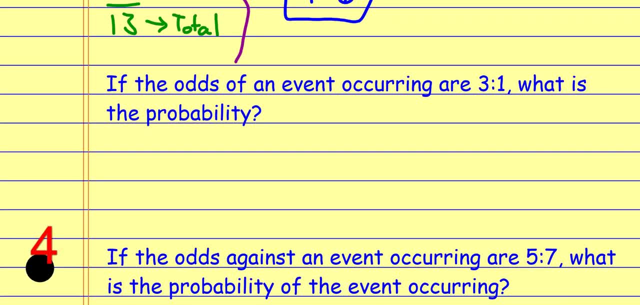 want. If I look at this one, it says the odds of an event occurring are three to one. Now, what's the probability? So again, start with odds. The odds are three to one, This is favorable And this is unfavorable, And so, in other words, there's three ways I can get what I want. 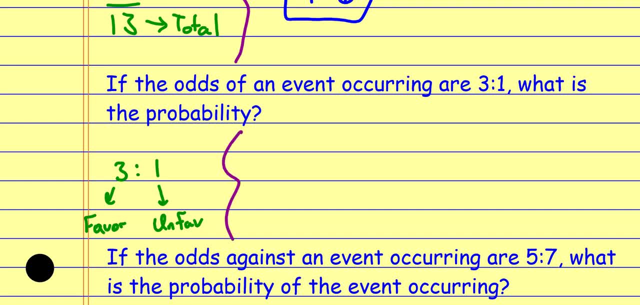 And there's one way that I could get something other than what I want. So when I think about probability, probability is the favorable, it's what I want, which is the three, but now over the total, And so start thinking about the total. If there's three good things that could happen, 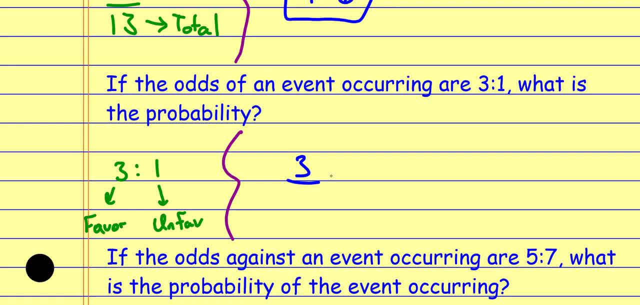 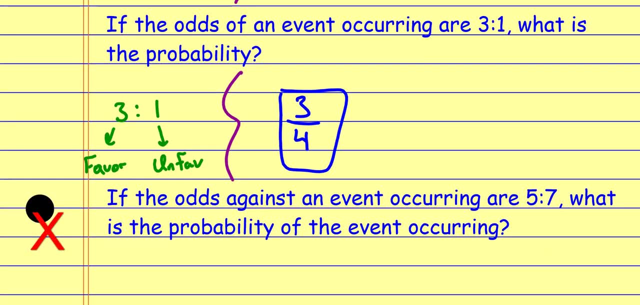 and one bad thing that could happen, there are a total of four things that could happen, So the probability is three out of four. okay, Again, there's a very slight difference between these things, but we want to make sure we understand the difference between on versus probability. If the odds against an event 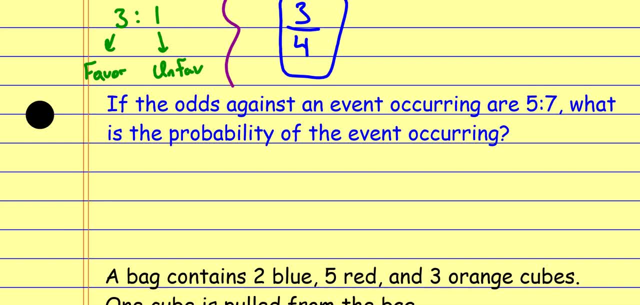 occurring are five to seven. what is the probability of the event occurring? So again, once again, just think about what odds means. So here's odds against the event, which means this is the unfavorable listed first, And then these are the favorable outcomes listed second. 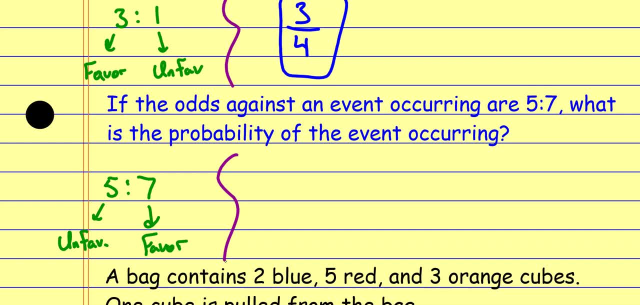 Okay, so now if I want the probability of the event, the probability of that thing happening is favorable over total. So looking at the odds, I can see the favorable outcomes would be seven. And now if there's seven ways I could get what I. 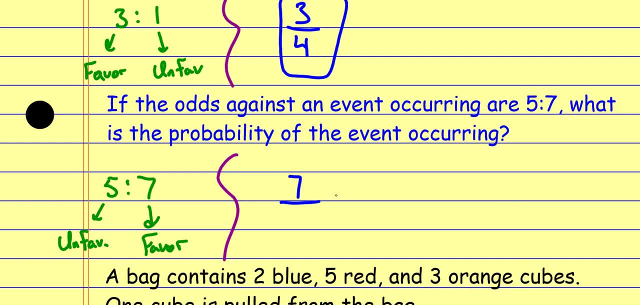 want. according to the odds, there's five ways that I could get something other than I want. That's a total of 12 different options, So it's seven out of 12, okay, And now kind of mixing all this together, just bouncing back and forth between the two. 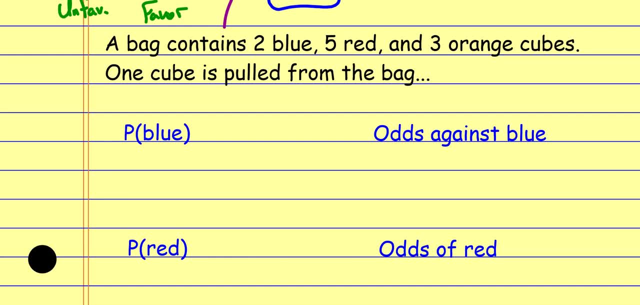 A bag contains two blue, five red and three orange cubes. One is pulled from the bag. What's the probability of blue? So the probability, remember, is what I want over the total. So there are two blue out of a total of 10 marbles, and that reduces to one fifth. 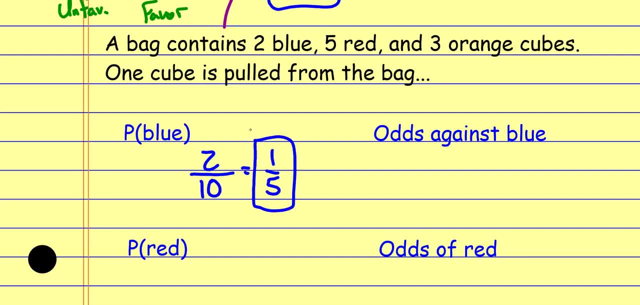 So that's the probability. okay, Odds against blue. all right. So there are two ways I could get what I want, which is the blue. There are eight ways that I could get something other than what I want, So in this case, I want to list the eight first. So it's eight to two, which, of course, 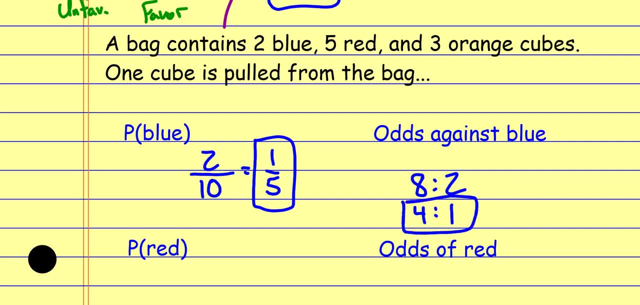 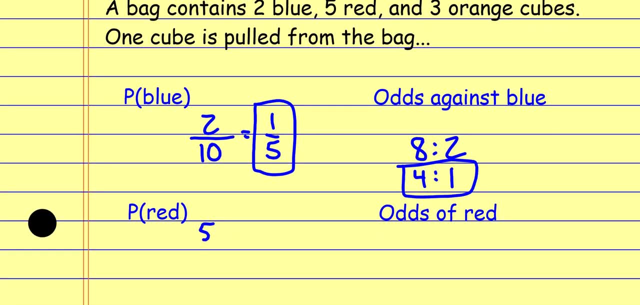 I want to rewrite as four To one. Okay, that's the odds, The probability of red, So there are five red out of 10 total, which is one half, And then the odds of red. there, once again, are five red, So there's five. 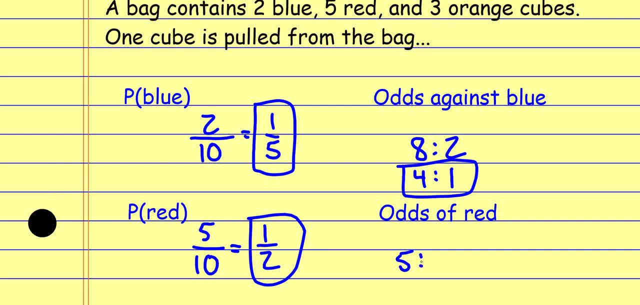 ways I can get what I want. But then, comparing that to the other stuff, there are five ways that I could get something other than what I want. So now the probability is one to one, or sorry, the odds are one to one. 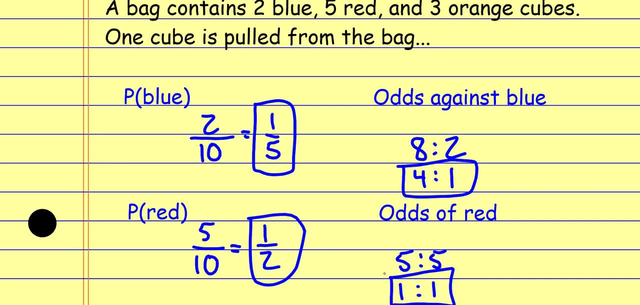 So again, that slight difference. Probability is what we want over the total, Odds are what we want versus what we don't want, And if we say odds against, we just switch it. It's what we don't want versus what we do want. okay, A very slight difference. They're similar but they're. different okay.